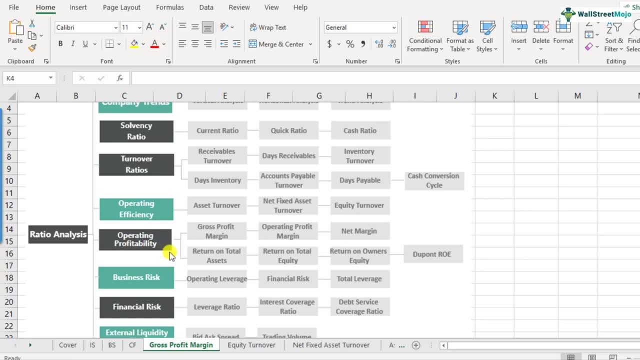 and it comes under the operating category. Here we will be discussing three margins, like the gross profit margins, operating profit margins and the net profit margins, But in this video we'll be discussing only one, that is, the gross profit margins. So, in order to fully understand what this margin is, it's divided into two parts. 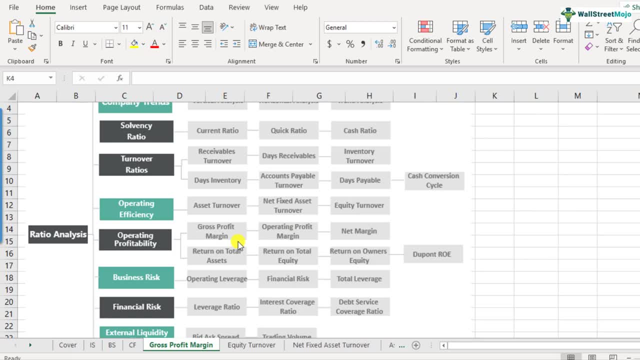 The first part is the gross profit and the other part is the sales. So what is gross profit? Gross profit is, let's say, as a company, if you've done any sales. so whatever is the cost of direct sales, the cost of direct sales? once you deduct that cost of direct sales you get. 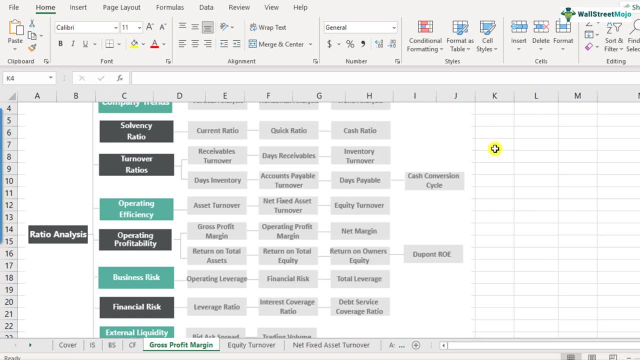 gross profit. So I'll explain- might have already explained- that within Laurick 20 00 00, that within help of an example, let's say you have done a sales of 1000.. So there would be cost of direct sales, like some costs will be associated with. 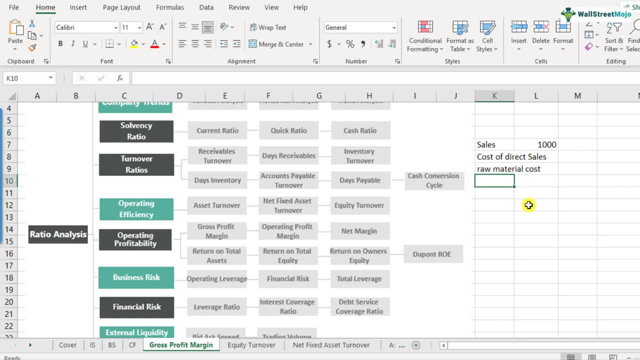 selling process, as well as procurement or raw materials. So what are the costs that can go under direct sales? it could be the raw material cost, Could be packaging costs, distribution cost, labor costs directly associated with that sales process will be the cost of direct sales. 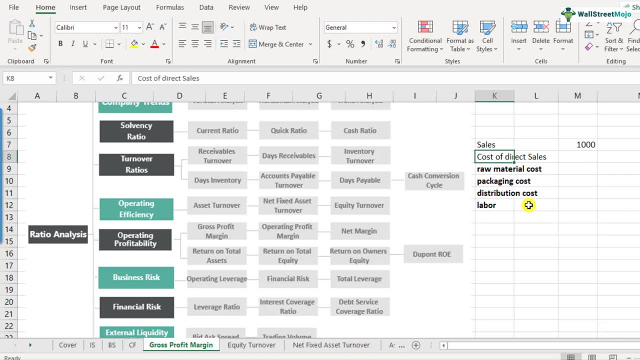 So if you have the sales as 1000 and let's say if your cost of direct sales is, let's say, 500, your gross profit is defined as sales minus the cost of direct sales. So that will come out to be 1000 minus 500, this is 500. 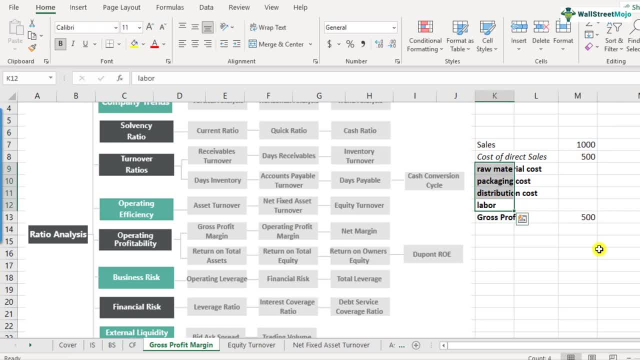 So any cost which is direct cost needs to be deducted and that will be called as cost of direct sales. We also call this as cost of goods sold- COGS. okay, so it is also called as COGS- cost of goods sold. So now that we know what is gross profit, the formula for gross profit margins is very 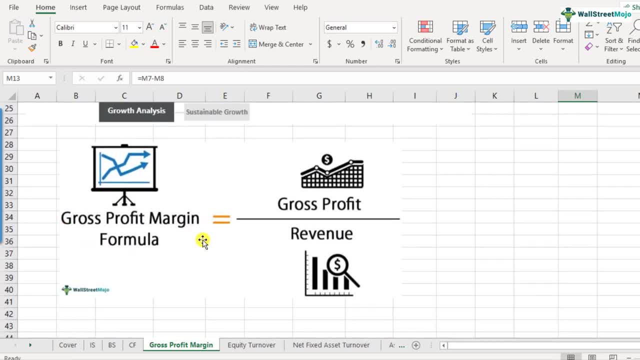 very simple. I'll show you the formula. The gross profit margin formula is gross profit, the one which we calculated just above and below the revenues. Revenue is nothing but the sales numbers. okay, So in this case, what do we have? 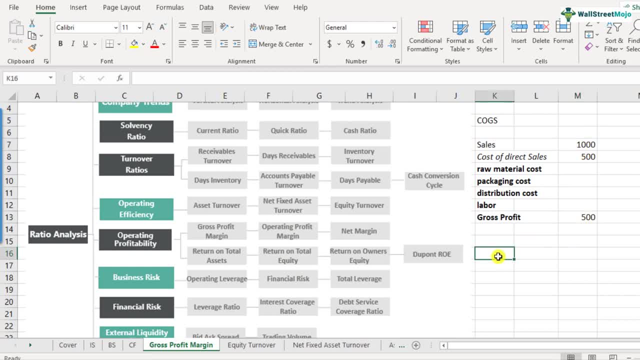 Sales as 1000 and gross profit as 500. So what do we have in terms of gross margins or gross profit margins? That comes out to be 500 divided by 1000, that is 0.5.. So when we convert this into percentages, we get this as gross profit margin as 50%. 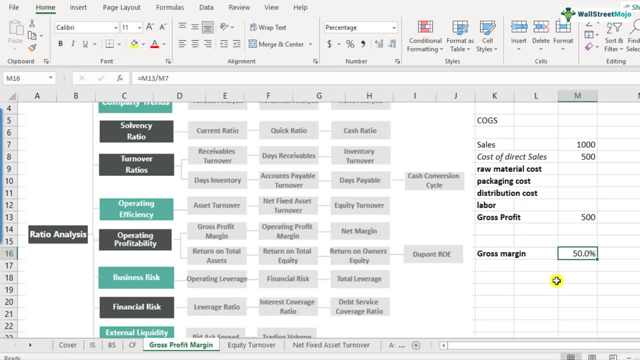 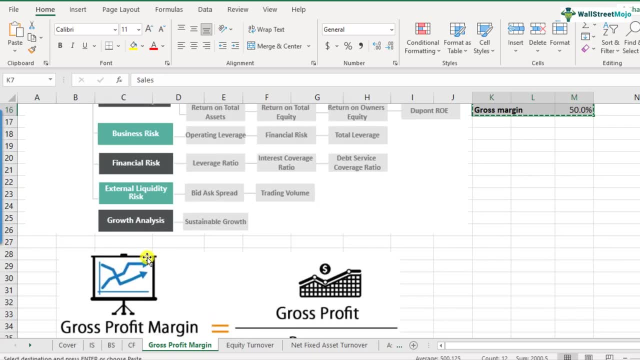 So that's how gross profit margin is calculated. Gross profit margins is actually calculated and its interpretations. we'll just look at it in a moment. Let us now look at some of the nuances of the gross profit margins. So I'll just copy the same example. 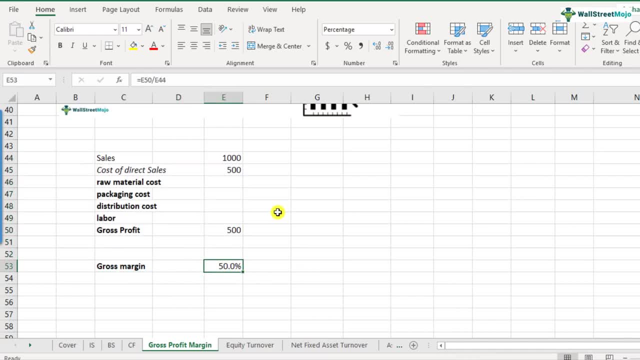 So where we got the gross profit margins here? So let's say there are two companies: This was company A and then there is company B. okay, Then there's company B That has gross profit margins of, let's say, 58.3%. 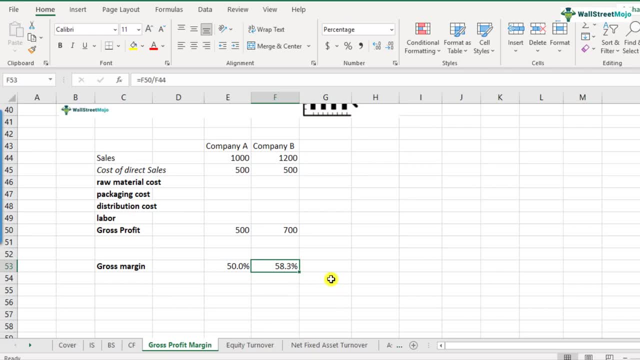 So what does it tell about? you know which one is better? Of course, the one that is generating higher gross profit margins will be better, right? So in this case, when we are talking strictly about these two companies, between company A and company B, company B is generating higher gross profit and therefore its results in. 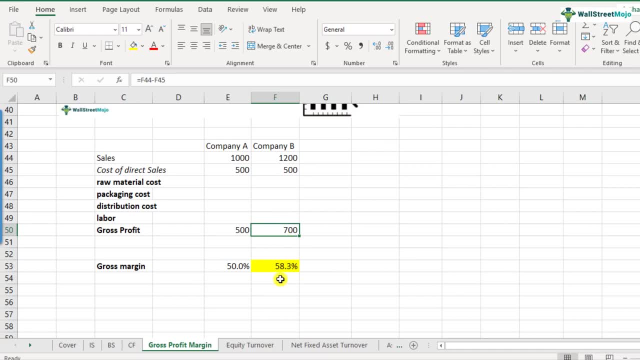 higher gross profit margins on a per dollar basis, Gross profit margins, Gross profit margins of company B is 58.3%, So that's much higher. Now, having said that, you need to be cautious about the fact that both these companies should be from the same industry. 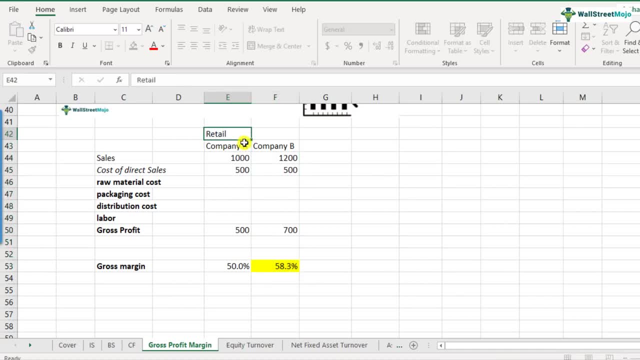 So you cannot compare. let's say this: company A is in retail and the company B is in automobile. You cannot say that company B is doing better and company A is not doing better because they are in the different, unrelated industries So they have to be in the same industry. All together. only then can you compare it right. So some of the industry where you will find the very high gross profit margins could be easily like hospitality, hotels, restaurants. These are the industries where you will find typically a higher gross profit margins somewhere. 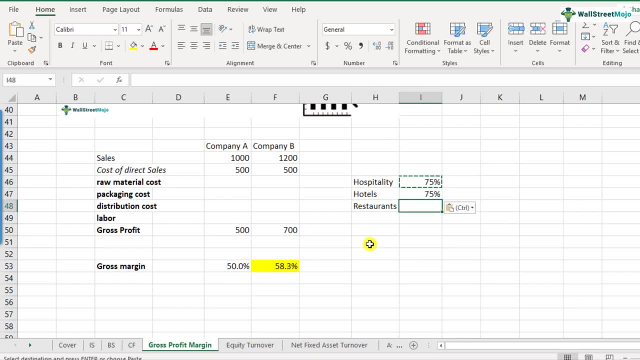 around 75%. maybe in restaurants it will be around 60, 65 odd percent. So this is typically higher Because you know, if you look at the way they are placed, the raw material cost for them is not high. 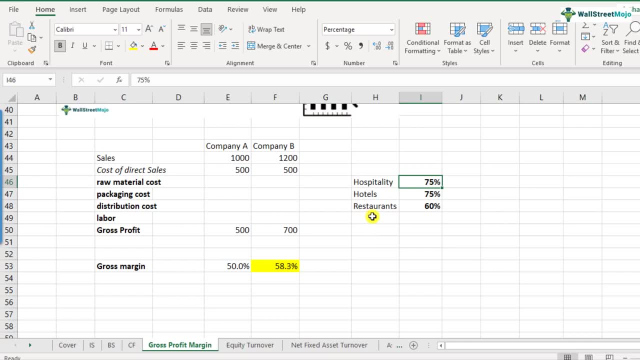 For a hotel industry. if you look at for a hotel, they've already invested a lot of money in building the hotel right, So for them the raw material is the extra cost which they have to bear when the customers check in right. 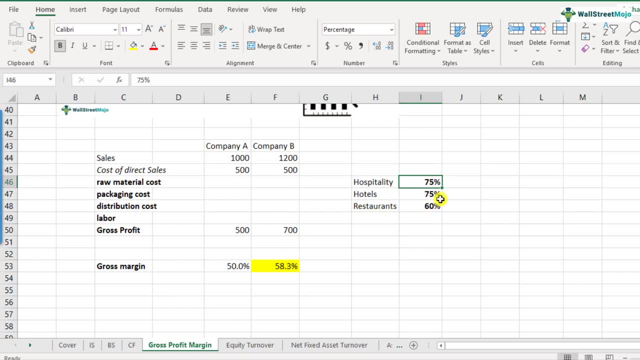 Or the food cost, etc. So that's why the gross profit margins for such industries is very high. Now compare this with, let's say, a hotel, Let's say another, for example retail or auto services, for example. you know they. 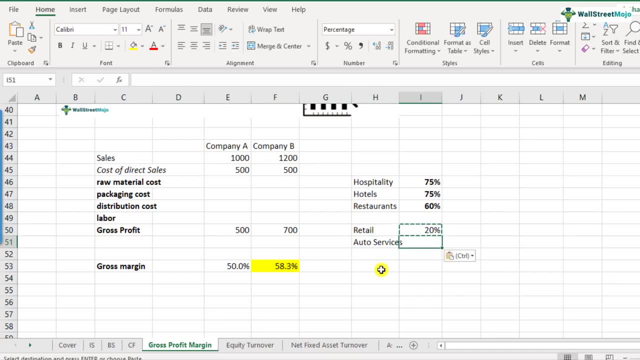 would not have a very high profitability margins. you know, somewhere around 20, 25 odd percent will be the gross profit margins for them, Because in this case what happens is that the raw material cost essentially is a very high cost altogether. 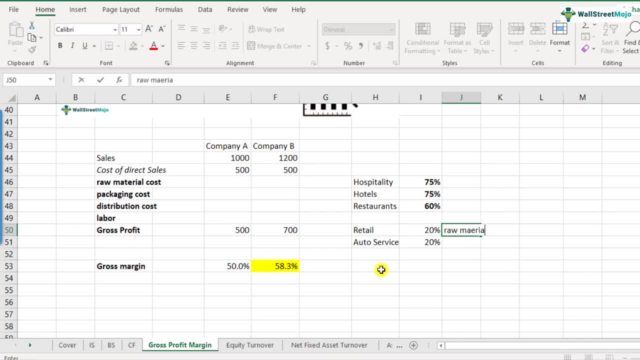 The raw material cost, you know the labor cost, Labor cost is kind of very high. So that's why the such industries actually show a very low gross profit margins. So that's, that's one thing which I wanted to actually share with you. 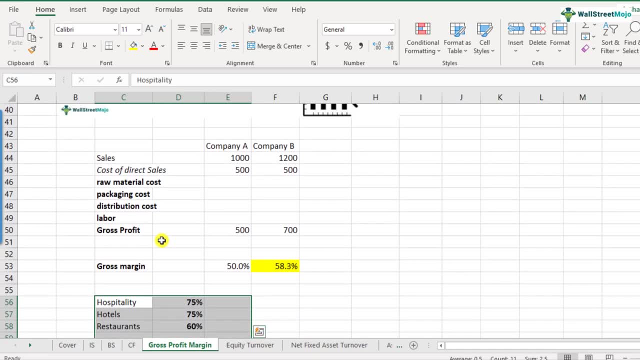 Another important aspect of gross profit margins is that you know sometimes when you look at the annual reports there are certain expenses which are not direct expenses, direct cost of sales. They're like indirect cost of sale. One example which you will definitely find in some of the annual reports is the depreciation. 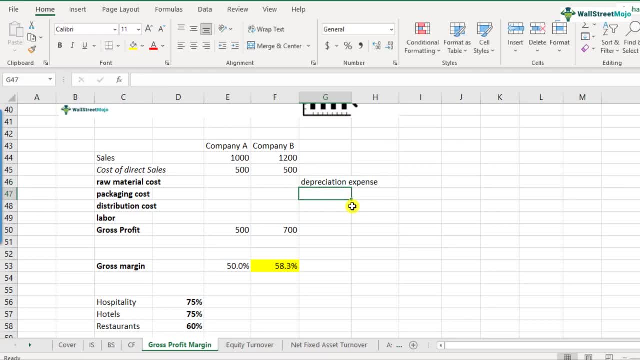 expense. Okay Now depreciation expense in some SEC filings is. I mean it's reported as a separate number, but in some of them it is actually included, So it's included in the cost of sales or it's also included in the purchasing cost. 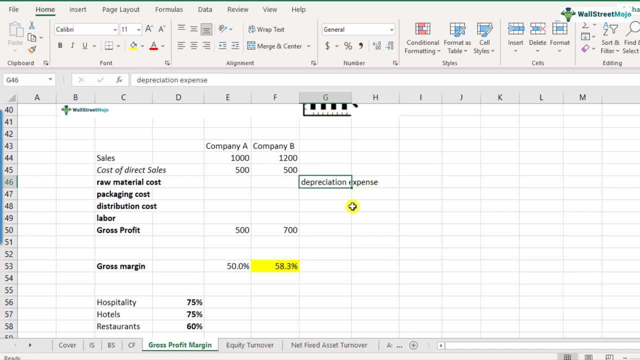 of the raw material cost. you know different types of costs, So you have to read through the annual report and find that out. Okay, So in this example, you know, I'll just remove the company B for the sake of convenience. 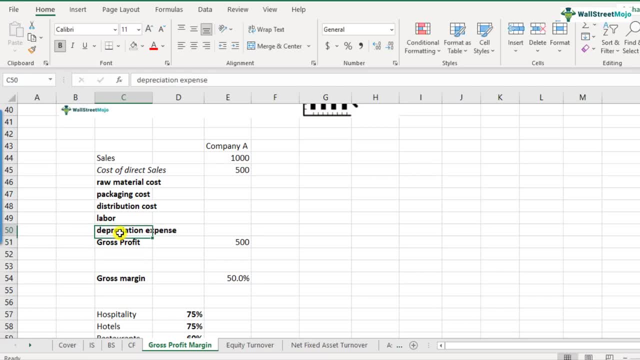 So let's say there is a depreciation expense which this company A has included, and that was a hundred. Okay, So this is the amount that was already included in the cost of sale. So 500 includes the depreciation expense. Now is depreciation expense a direct expense? 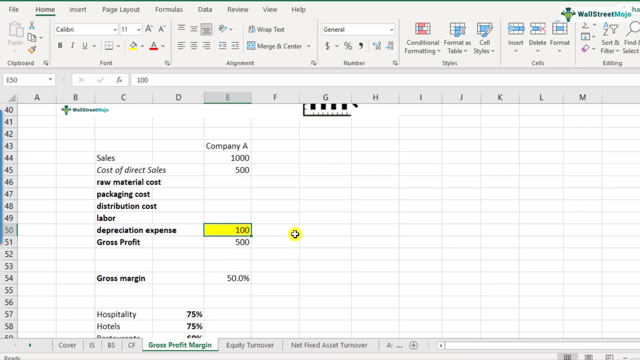 No, it is not a direct expense. Okay, It should be an indirect expense, It should come below gross profit, but it is because of the way the company has disclosed it. You know they have included it as a depreciation expense. So in this case, what you need to do here is you need to exclude this from cost of direct 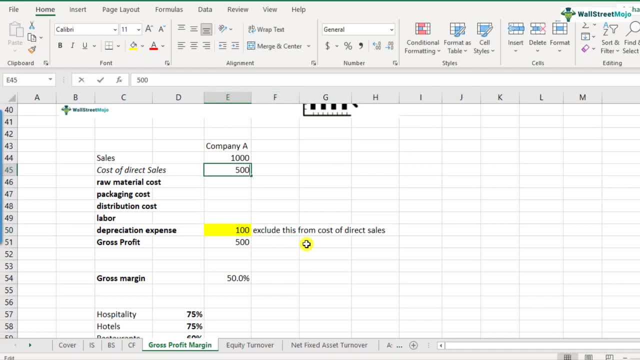 sales. Okay, So what this means is that your cost of direct sales was 500. that included the depreciation expense. You need to remove this hundred, So your cost of direct sales will become 500. And your gross profit then jumps to 600, because this is the correct picture. you know it. 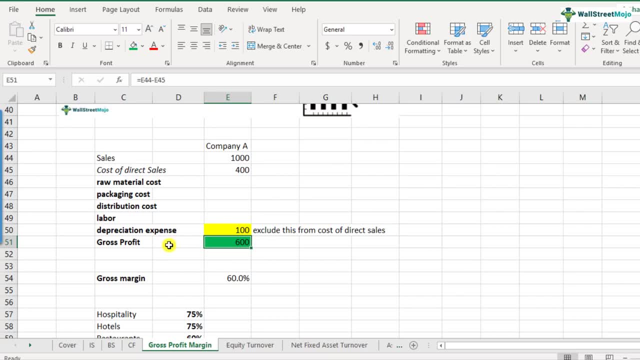 should not include the indirect expense. So that's why gross profit comes out to be 600 and the gross margin actually increases to 60%. So that's how you need to understand gross profit margin. So when you're comparing two, three companies and trying to understand what is the gross, 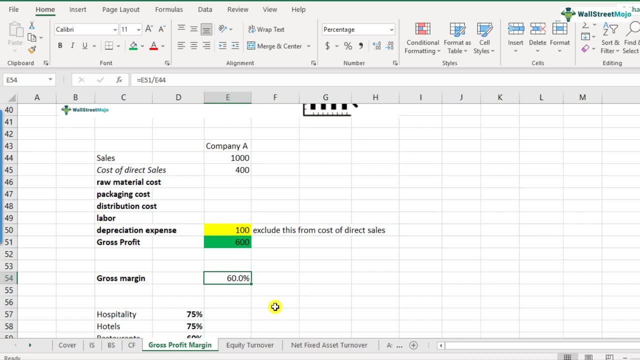 profit margins between the two. You need to also understand these subtle differences. Okay, Whether they are included or not. if they are, you have to exclude it from the calculations, All right? So I hope you understood what is the gross profit margins and why they are high or low. 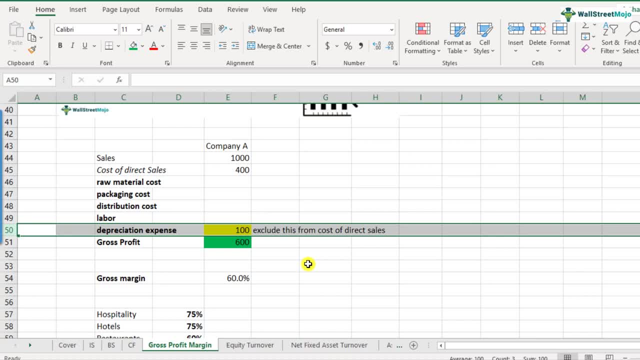 for some of the industries, and which kind of costs should be included and which could be should be excluded from the cost of direct sales or COGS. Now, having understood this, let's go to the Colgate case study and see what's its gross. 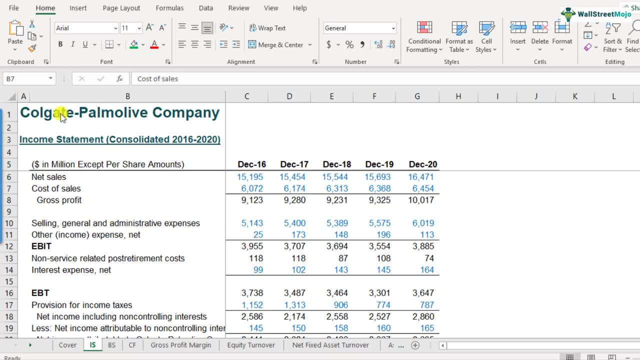 profit margins are all about. So here is the income statement of Colgate And we can see that, uh, within the income statement the company has provided net sales and the cost of sales and we also have the gross profit number. So we don't have to kind of calculate it from the figures. but yes, as I said, one thing: 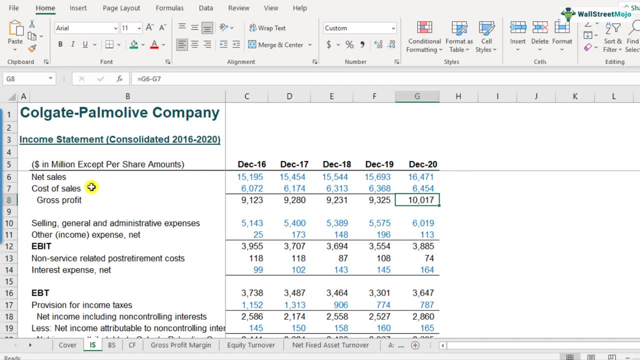 that we need to check is that whether cost of sales contains the depreciation or any other kind of indirect expense, And for that you need to actually go back and read through the SEC filings. All right, So that needs to be done, but for the sake of convenience let's come to the direct calculations. 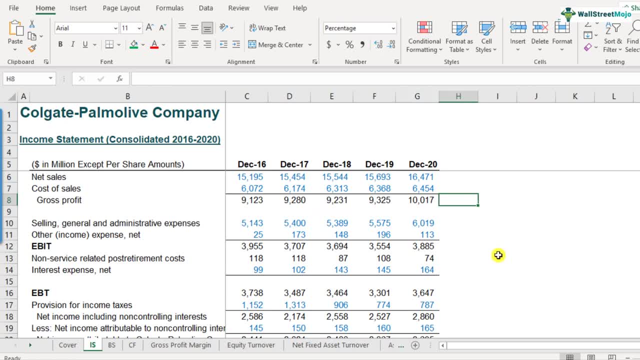 Here is the gross profit margin. So what is here? What is the gross profit margins? The gross profit margins, as we have defined earlier, was gross profit divided by your sales, or net sales, or revenue. All of them are like one in the same. 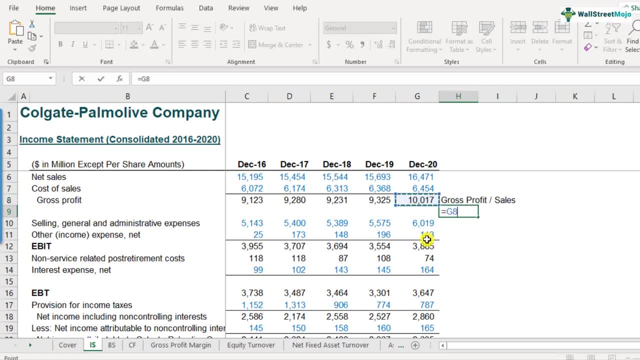 So here this will be: gross profit is 1 0, 0, 1, 7 divided by 1, 6, 4, 7, 1.. So that comes out to be, in percentage terms, 60.8%. okay, That is for December 20.. 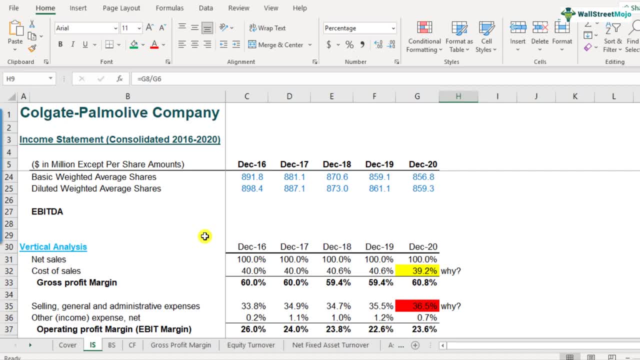 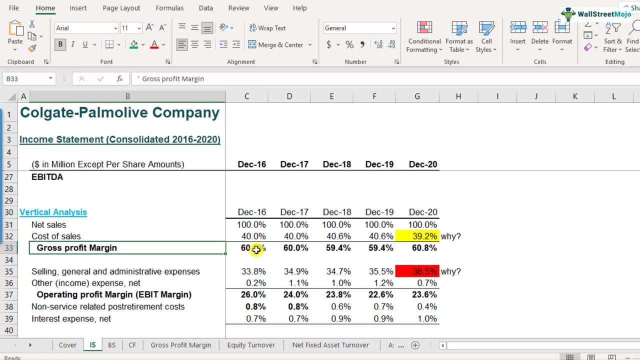 Okay, So if you scroll down, actually we have done this already. We did this vertical analysis, You remember, in one of the videos and where we did calculate the gross profit margins. So this, if you look at the historical trends, we note that the cost of sales is around 40,. 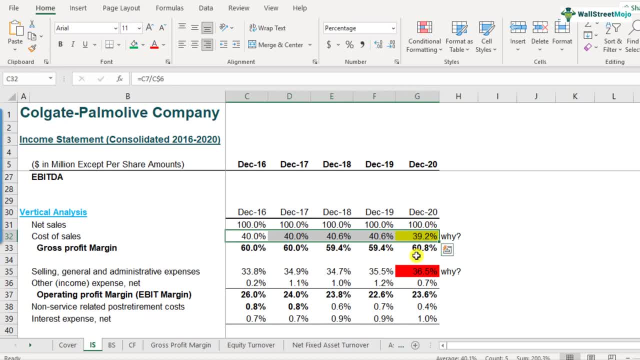 40, 40%. you know, more or less it's in the range of 40.39.2 was the most recent, but it's more or less in the range of 40%. And then we note the gross profit margins. 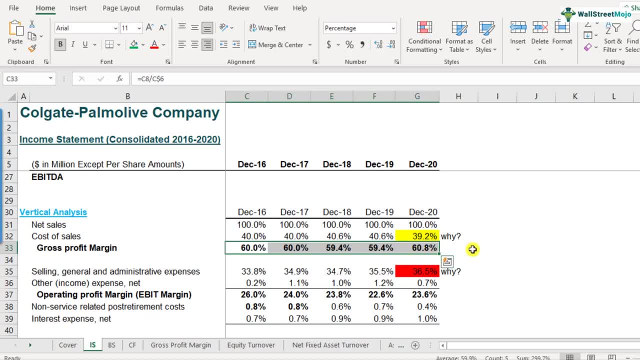 It's again more or less in the range of 60, 61%. as such, So the gross profit margins of Colgate has been fairly stable, And if we compare this with Procter and Gamble, we note that in Procter and Gamble the profit 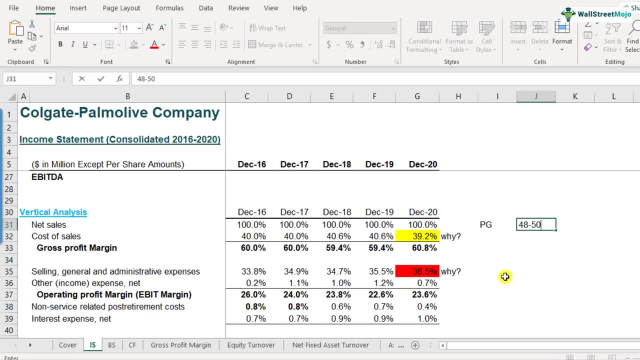 margin is somewhere around 48 to 50%. That's how their profit margins look like. So the gross profit margins comparatively for Colgate are much better as compared to Procter and Gamble. So this is how you can kind of interpret uh gross profit margins and calculate gross. 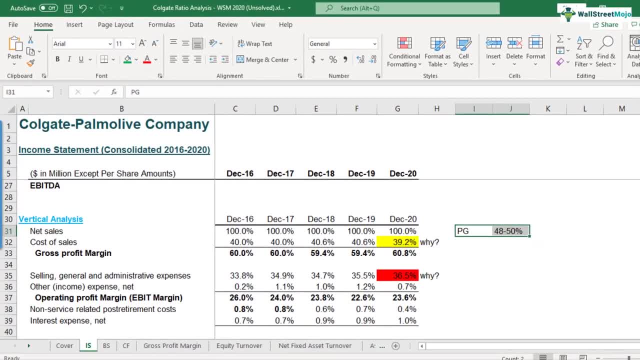 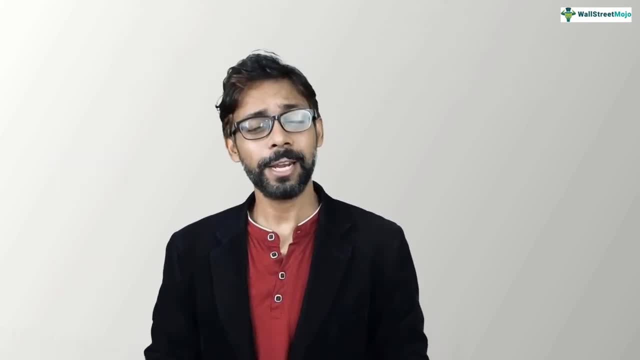 profit margins, And I hope you understood this as well. I hope you found this video to be useful. please do like and share, And if you have any feedback or want to suggest a topic for any future video, then you may do so by writing about it in the comment section. 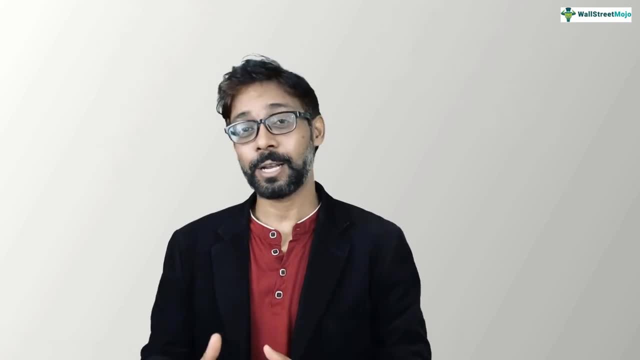 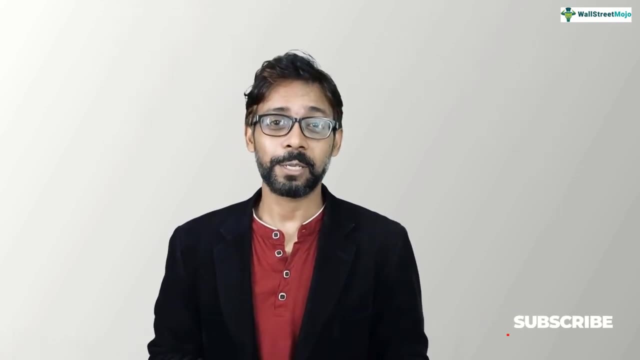 Also, we come up with very interesting videos on investment banking and core finance topics regularly, So if you haven't subscribed to our channel yet, then please do so by clicking on the subscribe button below, so that you can get the notification about our latest videos as soon as we release one. I hope you enjoyed the video. Have a nice day, Thank you. 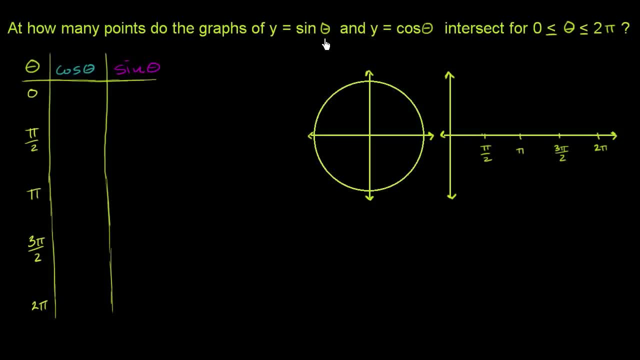 We're asked: at how many points did the graph of y equals sine of theta and y equals cosine theta intersect for theta between 0 and 2 pi, And 0 is less than or equal to theta which is less than or equal to 2 pi.